Click here to subscribe to Las Estrellas. the American New entertained. If you liked this video, be sure to be infected by the subscribe button. See other videos about African Americans and not just Americans. Guys, thanks in the big box. Happy Thanksgiving. 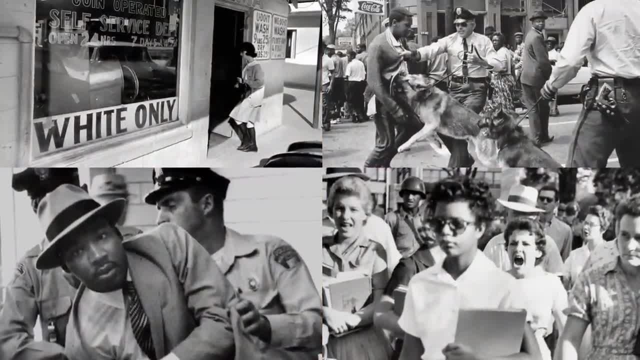 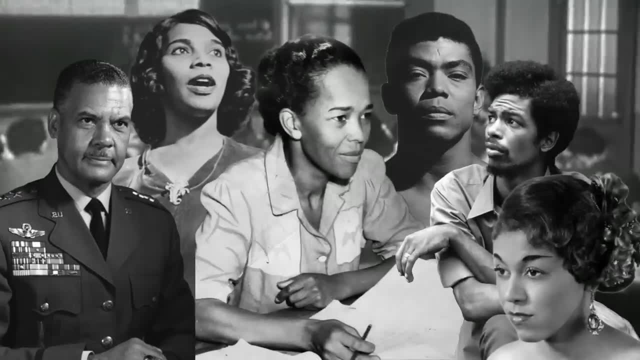 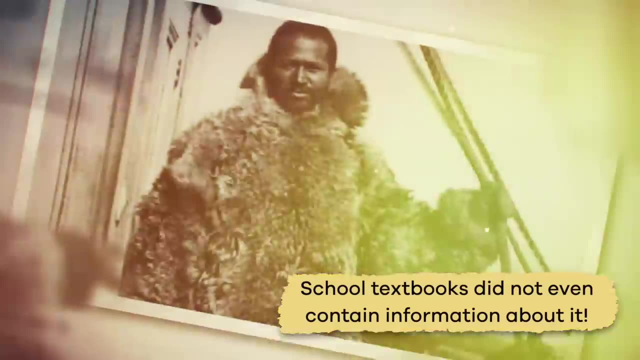 You will also get to know some of our next runs. slavery was officially abolished in the United States. racism and inequity continued Because of this as the years went on. few people studied black history. School textbooks did not even contain information about it. 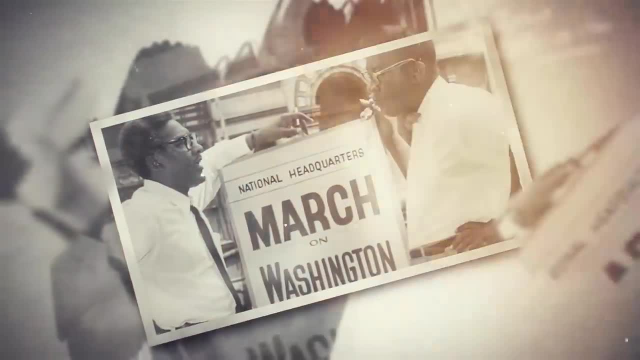 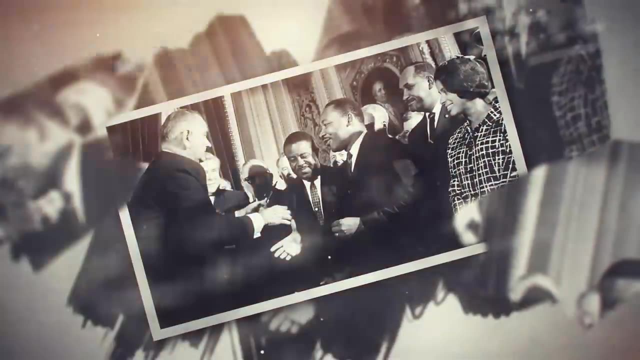 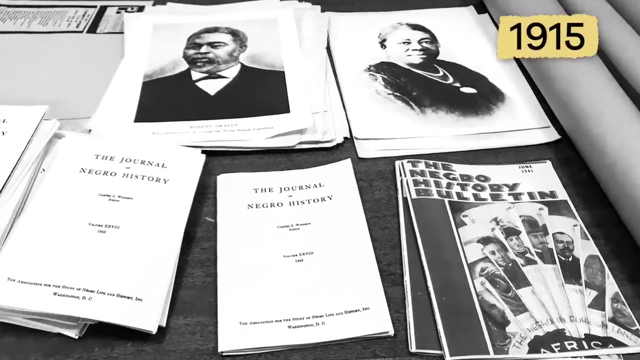 Can you imagine having a whole section of history left out of one of your textbooks on purpose? You would miss out on learning a lot of important information that you should know. Something needed to change In 1915, an African-American historian named Carter G Woodson made it his mission to begin. 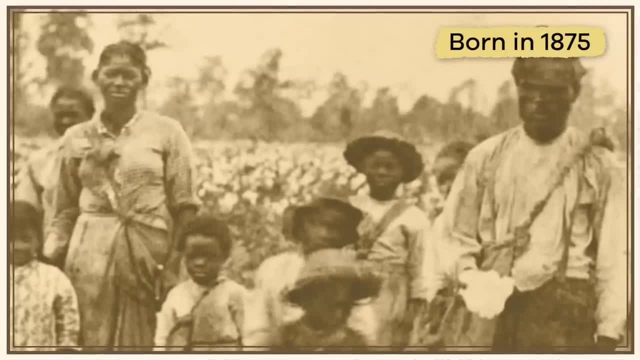 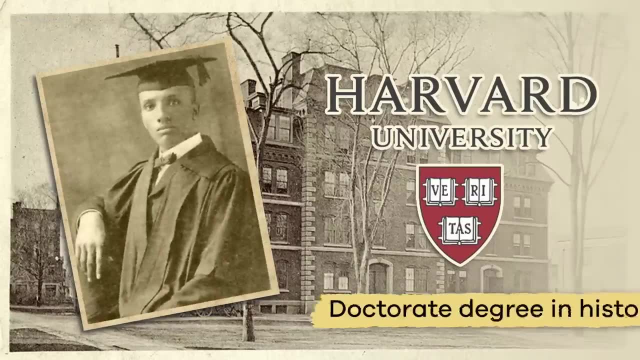 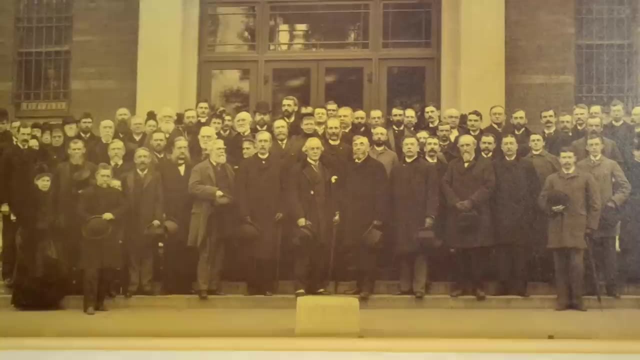 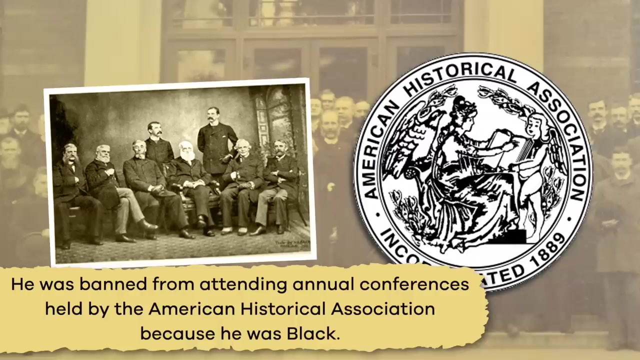 to document black history. Born in 1875 to formally enslaved parents, Woodson graduated from Harvard University with a doctorate degree in history. He became a faculty member at Howard University. While there, he was banned from attending annual conferences held by the American Historical Association because he was Black. He realized 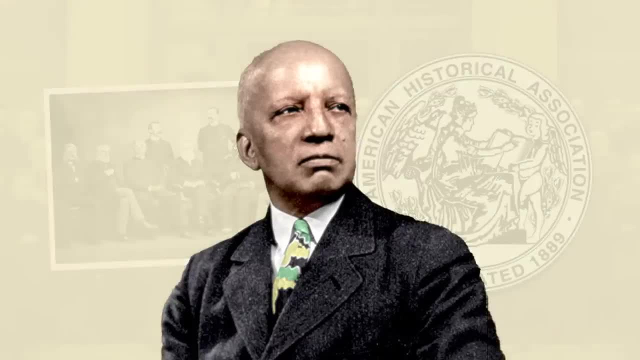 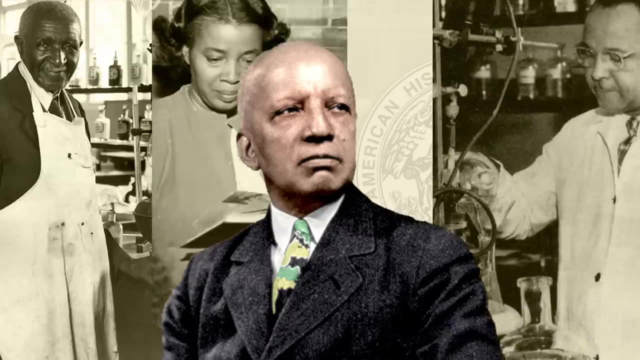 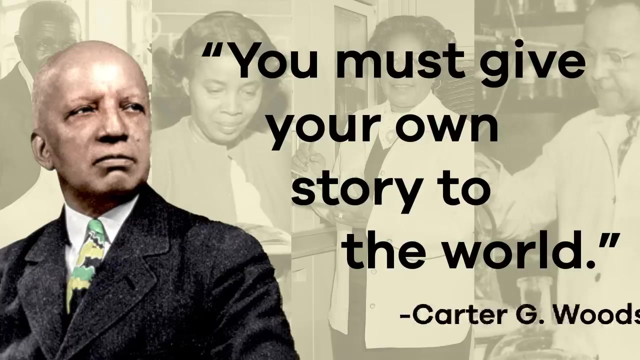 that the Mostly White Historical Association had no interest in giving Black people credit for advances in science, technology, education, engineering and other fields. Woodson wrote: you must give your own story to the world, And that is what he tried to do In 1926,. 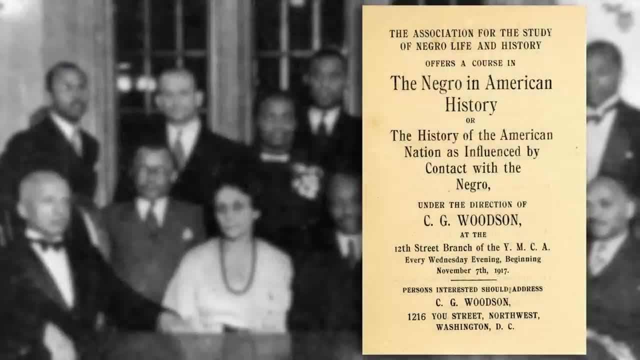 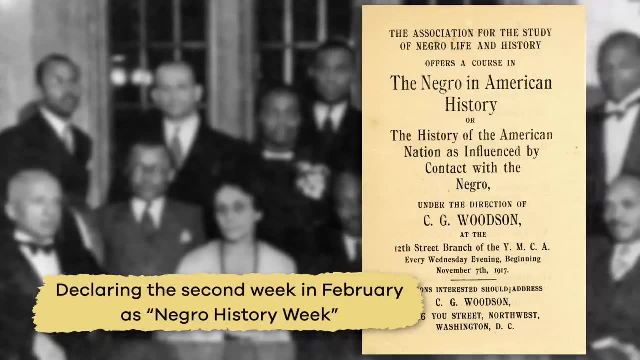 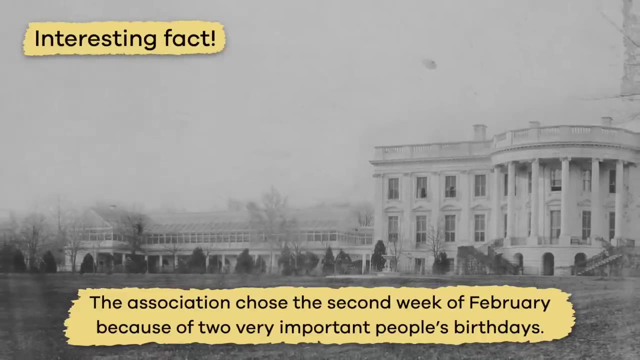 Woodson started the Association for the Study of Negro Life and History, declaring the second week in February as Negro History Week. Here is an interesting fact: The association chose the second week of February because of two very important people's birthdays: Frederick D Woodson and Frederick D Woodson. 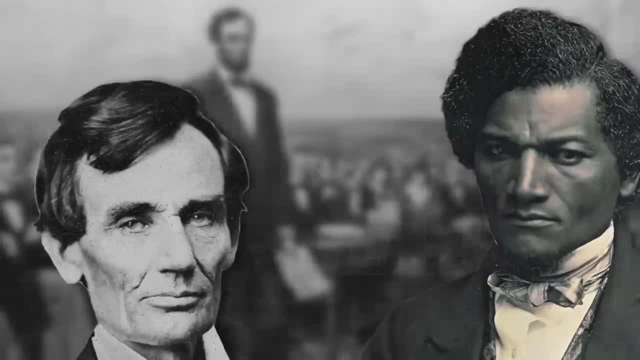 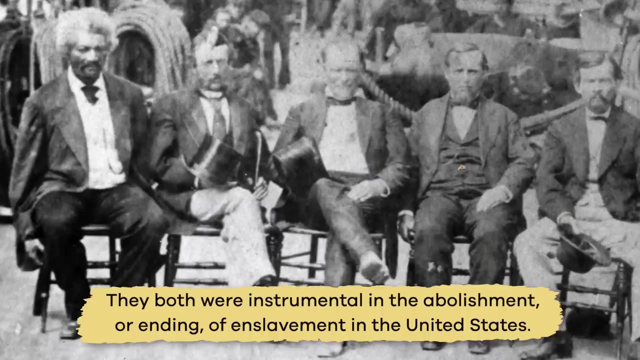 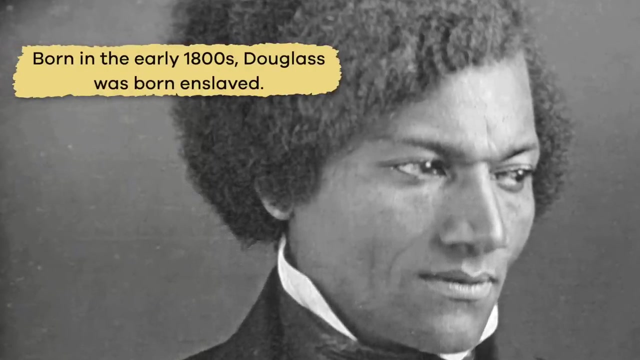 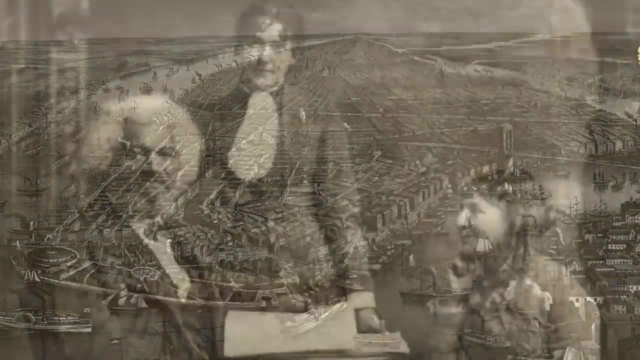 Douglas and Abraham Lincoln. Why these two? Well, they both were instrumental in the abolishment or ending of enslavement in the United States. Born in the early 1800s, Douglas was born enslaved but escaped to New York City in 1838.. He became an abolitionist, meaning he wanted to end the